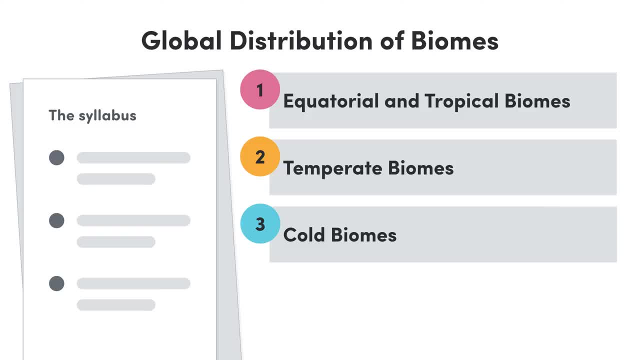 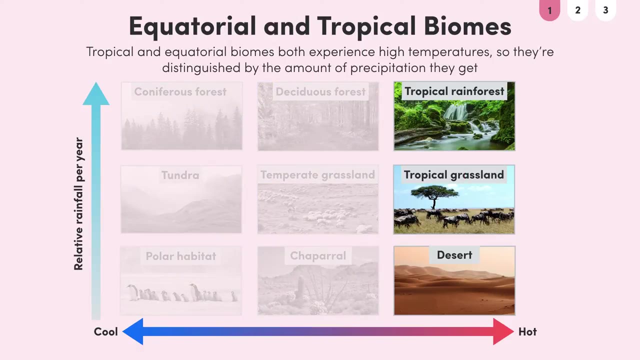 like and their characteristic plant and animal species. The biomes we'll cover are equatorial and tropical biomes, temperate biomes and cold biomes. So let's get started. Tropical and equatorial biomes all experience high temperatures, so they're distinguished by the amount of 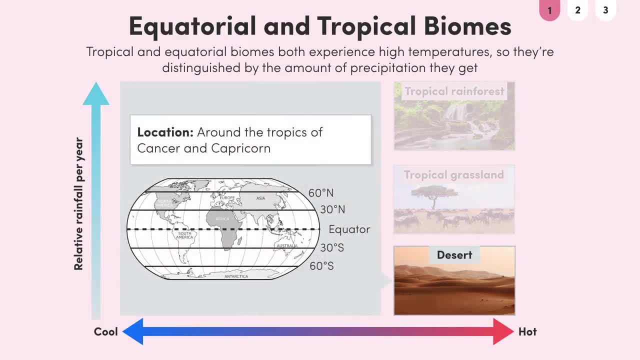 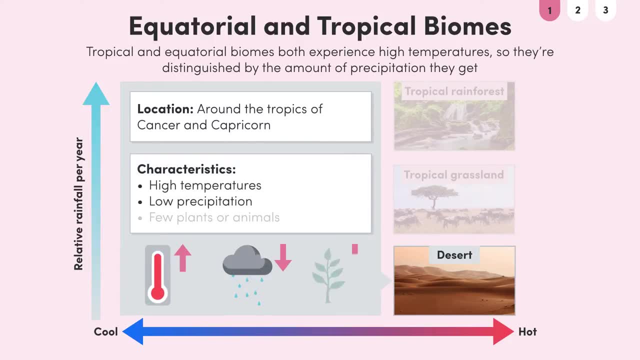 precipitation they get. Desert biomes are generally found around the tropics of Cancer and Capricorn. They are characterised by high temperatures and low precipitation, with very few plants or animals. The Sahara Desert is a great example of a classic sandy desert. 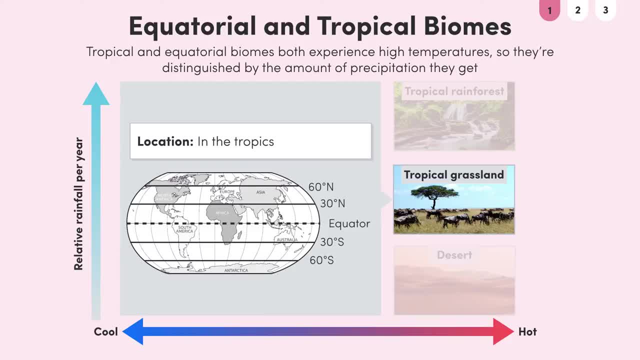 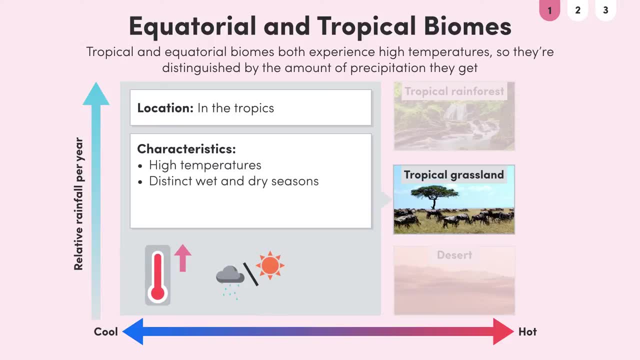 Tropical grassland biomes, also known as the savannah, are found in the tropics. Their climate is characterised by high temperatures, with distinct wet and dry seasons. The plant life consists mostly of grass with few trees. The African savannah is one of the 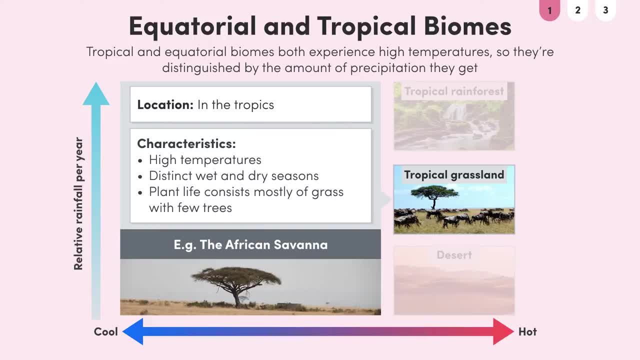 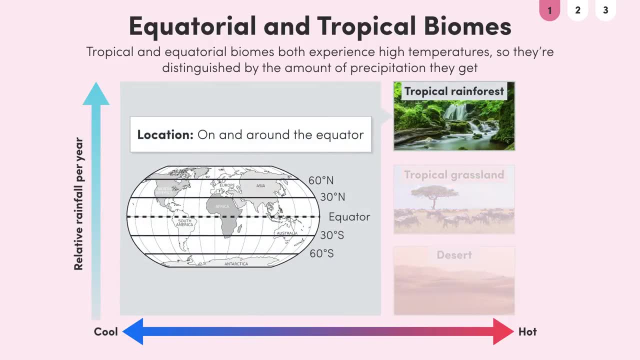 most well-known examples, but tropical grasslands are also found in Asia, South America and Australia. Tropical rainforest biomes, such as the Amazon rainforest, exist on and around the equator, where temperatures are high year round and precipitation is also high. 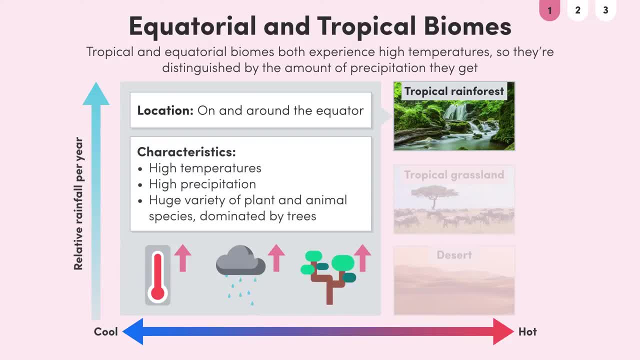 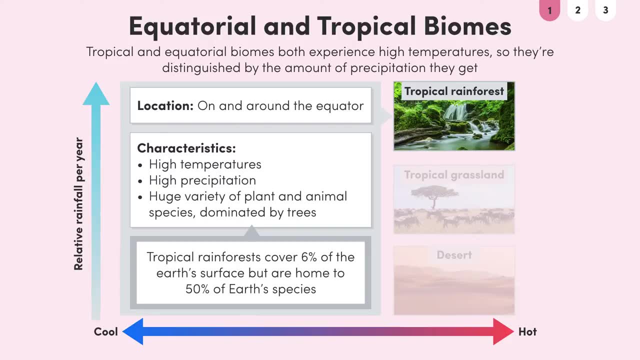 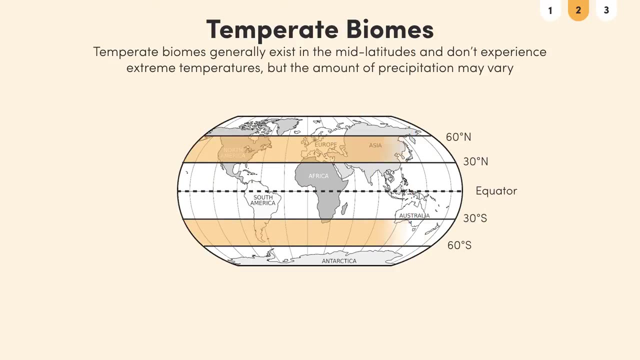 They have a huge diversity of plant and animal species. dominated by trees, Tropical rainforests cover only 6% of the earth's surface, but are home to 50% of the earth's species. Temperate biomes generally exist in the mid-latitudes and don't experience extreme. 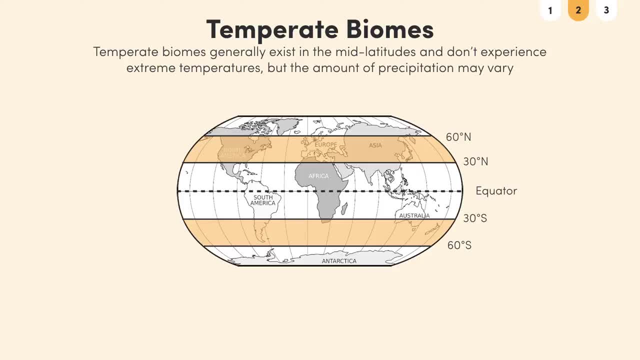 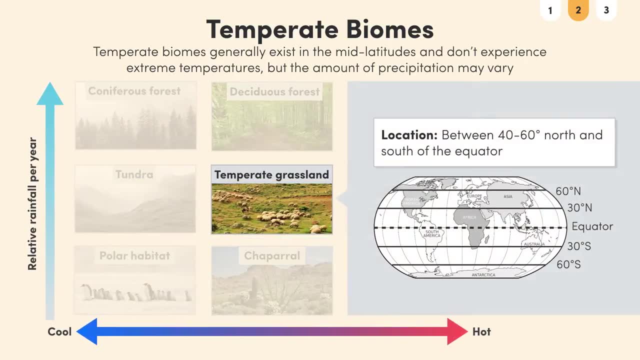 temperatures. although the amount of precipitation they get can vary, They usually experience four distinct seasons. Temperate grasslands lie between 40 and 60 degrees north and south of the equator, at higher latitudes than tropical grasslands. Like tropical grassland, 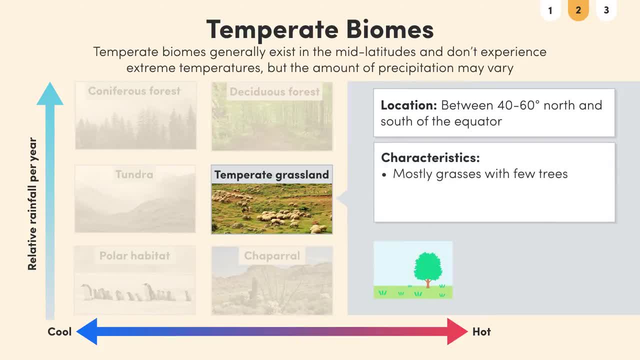 temperate grassland is also made up of mostly grasses with few trees. The climate is generally warm in the summer and cold in the winter, with minimal rainfall. The North American prairie is a perfect example of this biome. The North American prairie is a perfect example of this biome. 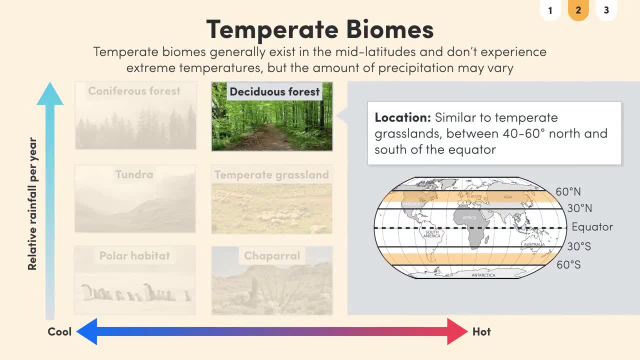 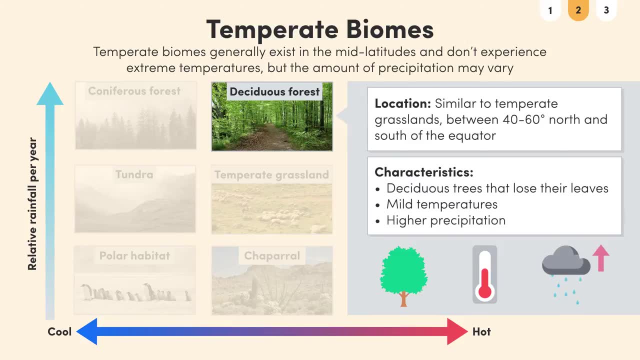 as it is called, the Murpwey and Bahrain Deciduous forest biomes lie at similar latitudes to temperate grassland and are made up of deciduous trees that lose their leaves. However, the temperature is milder and precipitation is higher than temperate grassland biomes. 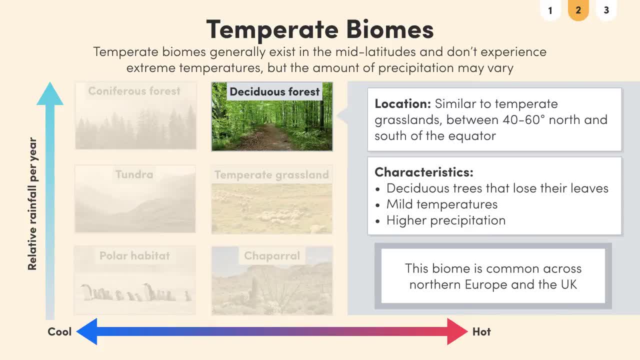 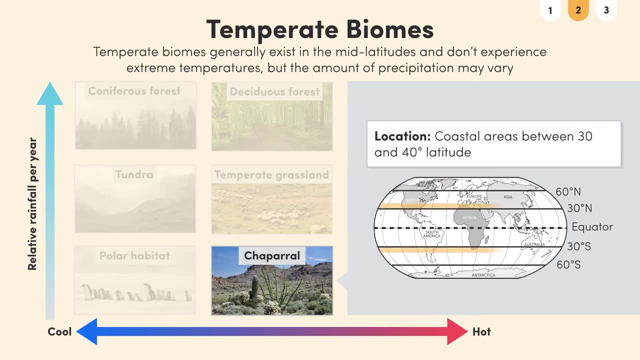 These biomes are common all across Northern Europe and the UK. Mediterranean biomes, also known as chaparral, occur in coastal areas between 30 and 40 degrees latitude. The plant life is mostly scrub and bushes that are adapted to the temperature of the forest. They also have the ability to bear fruit and, as you can see in this video, they also have the ability to bear fruits. Nuisance is a major factor that does not require a native plant to live on disputed lands. while there are those that can survive in theousy, It is definitely difficult to plant trees in the area of Oklahoma. 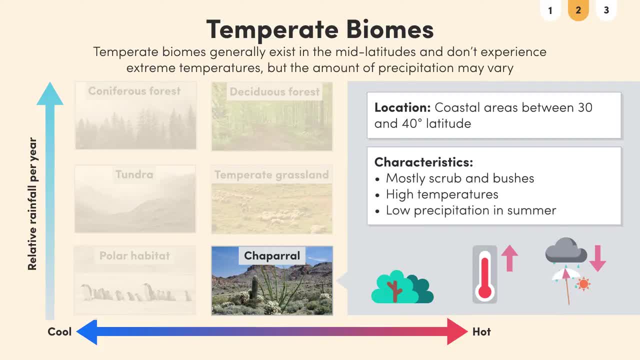 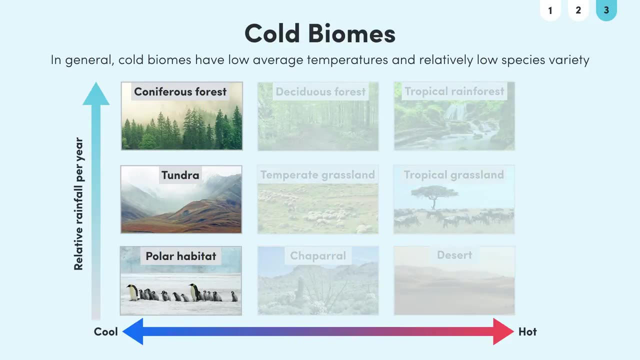 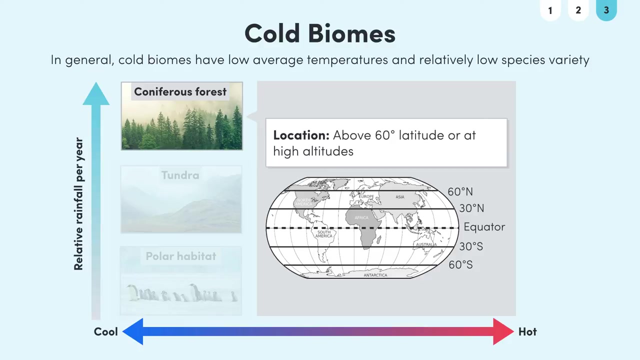 scrub and bushes that are adapted to high temperatures and little precipitation in the summer. As you might expect, this biome is mostly found around the Mediterranean, in places like Italy and Greece, So in general, cold biomes have low average temperatures and relatively low species diversity. Coniferous forest biomes, also known as tiger or boreal forests. 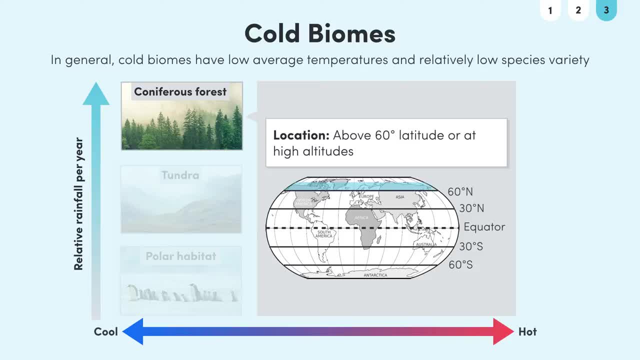 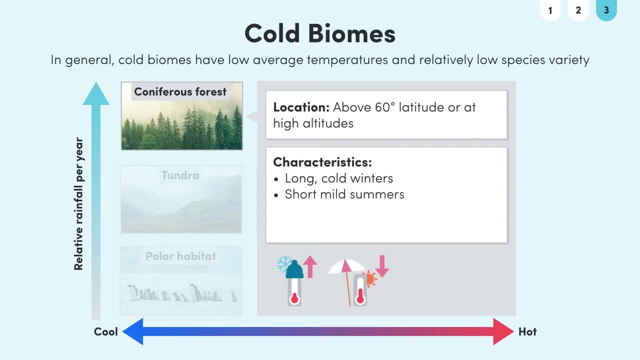 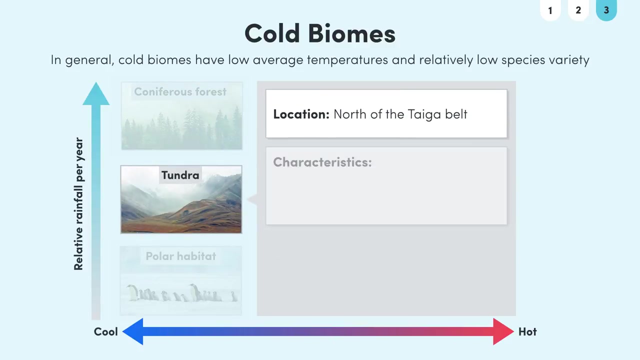 are generally found above 60 degrees latitude or at higher altitudes. The climate needed for these biomes consists of long cold winters and short mild summers with minimal rainfall, and the plant life is dominated by evergreens such as pine trees. Tundra biomes occur north of the Tiger Belt. The climate is so cold that the soil is permanently. 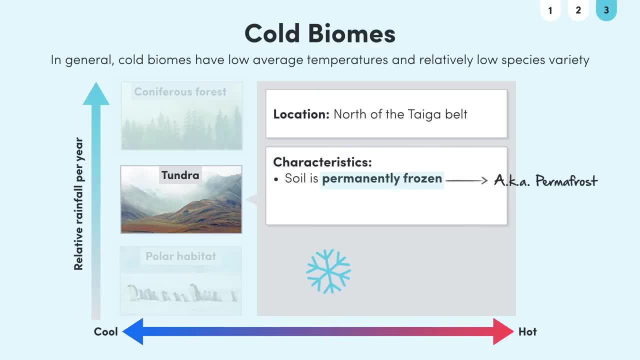 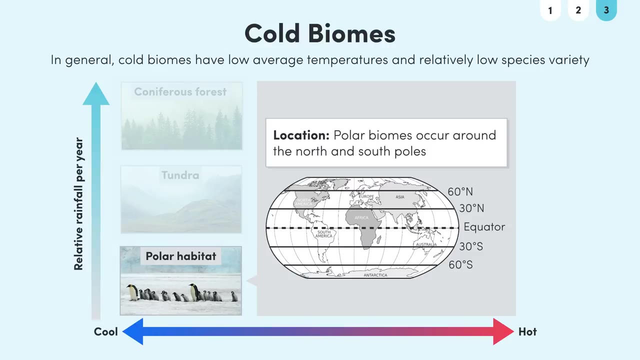 frozen, which is known as permafrost. Because of the permafrost, only mosses, lichens and some grasses can grow there. Tundra and tiger biomes are found across the far north of Canada and Russia. Finally, polar biomes occur around the North and South Poles. Only some mosses and lichens can grow. 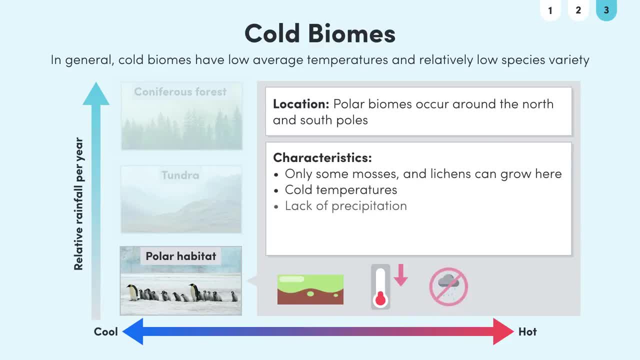 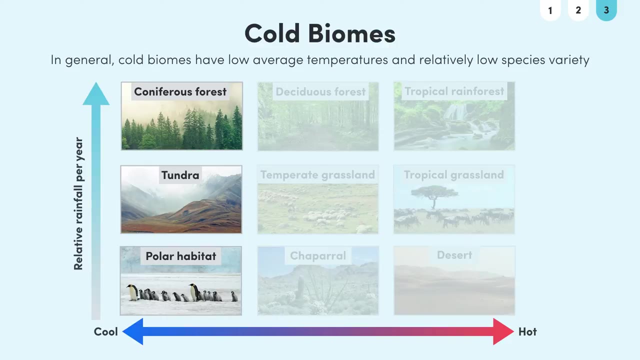 here. due to the very cold temperatures and the lack of precipitation, Often the land is covered in a permanent or semi-permanent layer of ice. The Antarctic is a perfect example of this biome type. But before we wrap up our cold biomes, there's one more that doesn't neatly fit into our diagram here. 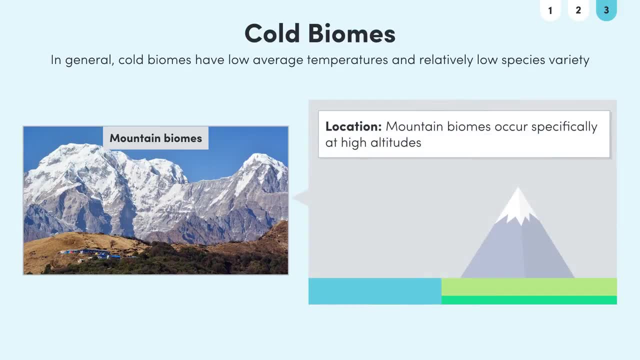 Mountain biomes. These occur specifically at high altitudes. They don't fit neatly onto our diagram because they're characterised by altitude rather than temperature and rainfall, but generally they're colder and receive higher rainfall than the surrounding flat areas, Because temperatures